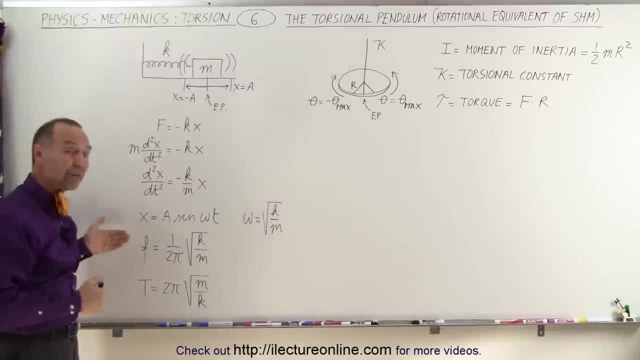 divided by the mass. We could then write the frequency of oscillation as such, which is 1 over 2 pi times omega. Omega, of course, is the angular frequency, which then becomes the square root of k over m, and if we then take the inverse of that, the period which is 1 over f, that is equal to 2 pi. 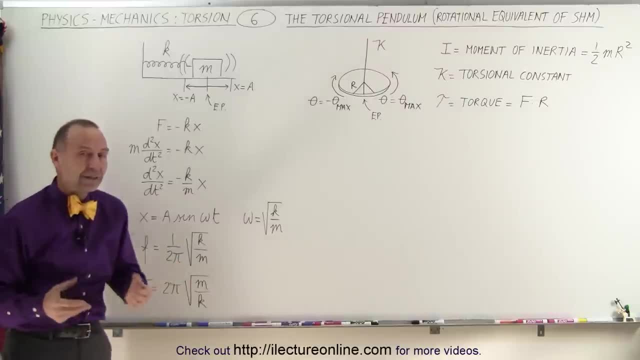 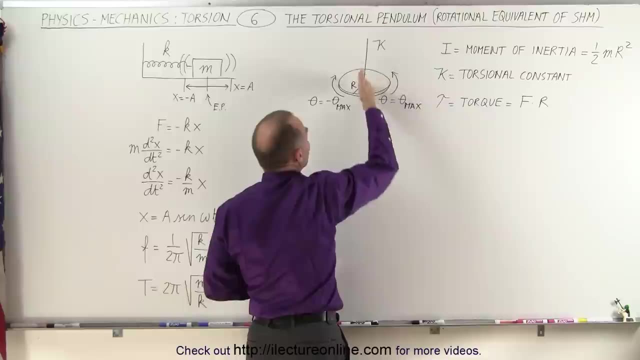 times the square root of m over k. Now we can have the exact same equations for a torsional pendulum. This, the string here, or the rod, whatever this is suspended on, will twist as you bend this back and forward, as you rotate it back and forth. 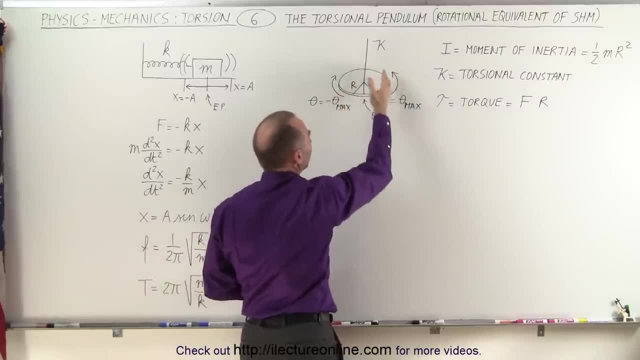 If we apply a force parallel to the side of the disc here, applying a torque, that will then twist this cable or twist this rod, and then we'll get it to go to its maximum displacement, the maximum twist angle we let go, and then this disc will then start rotating back and 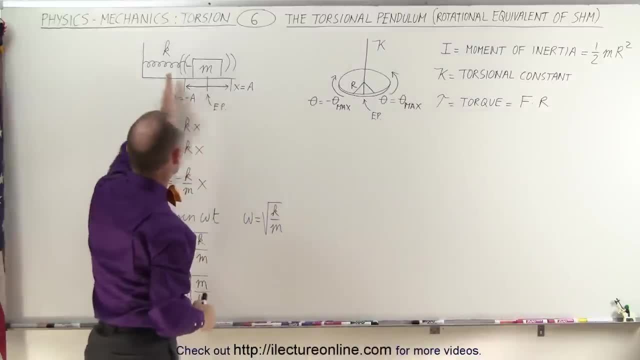 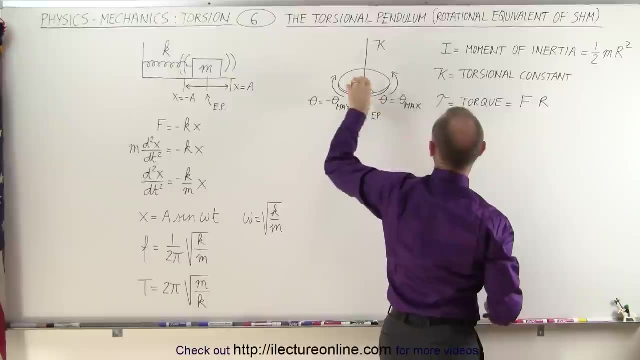 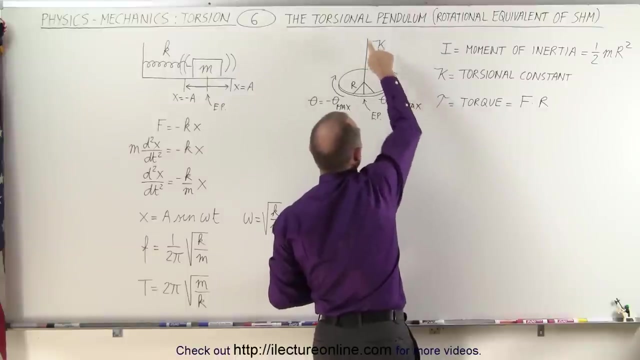 forth and back and forth, just like what we have here, with the mass going back and forth like this- Notice that i is representative of the moment of inertia- of a flat disc which is one half the mass times. the radius squared k is the torsional constant of this string or this rod or this wire. 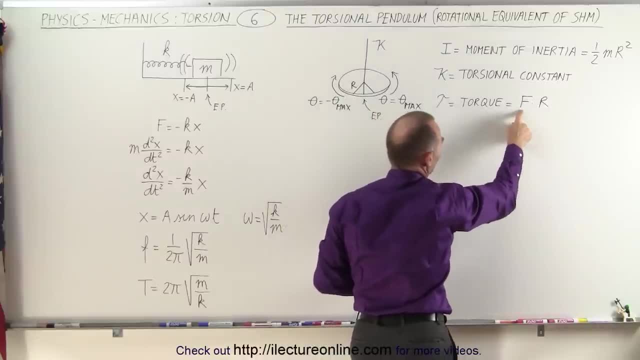 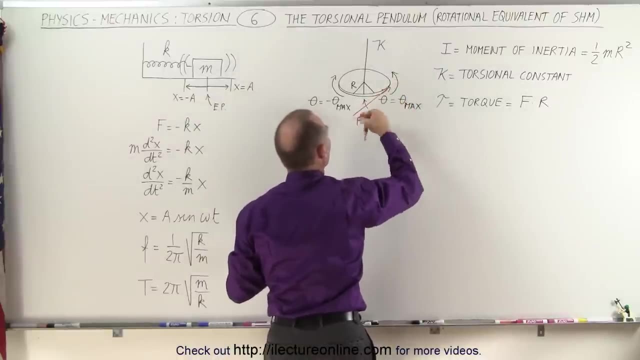 and here torque is defined as the product of f times r, the force applied to the side times r. Let me just go ahead and show you the force. so you're applying a force like this parallel to the edge that causes the disc to rotate. Now we're going to write the same. 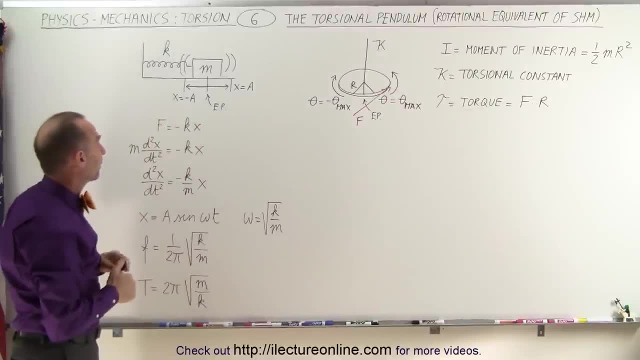 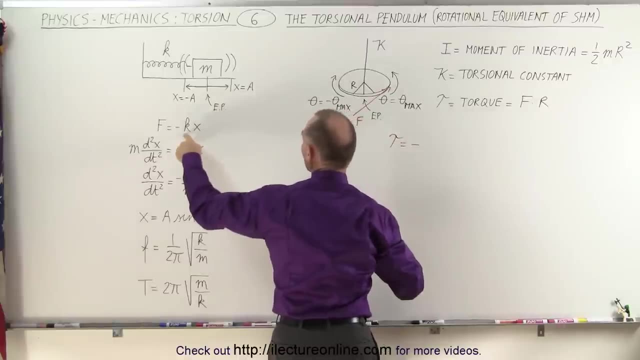 equations. but now in terms of rotational motion, like that, Instead of f, we write the tors. Torque applied to this disc will be equal to the negative. instead of the k of the spring constant, we use the torsional constant, kappa times. instead of the linear displacement x, we use 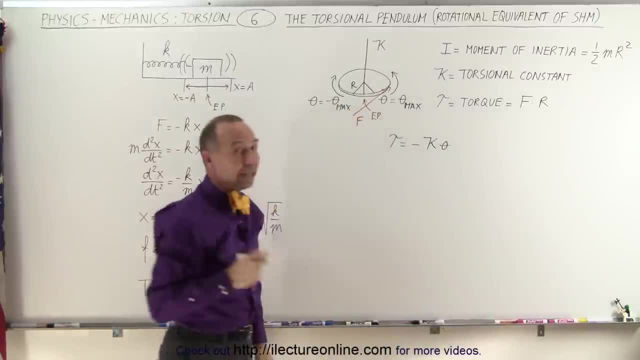 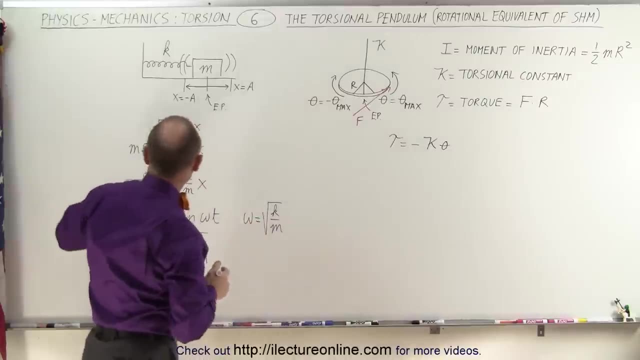 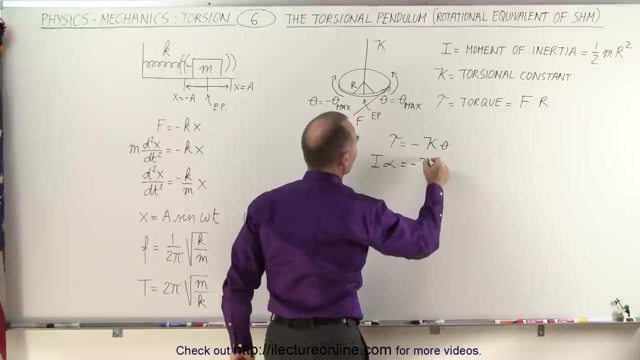 the angular displacement theta. We then realize that when you apply a torque, that causes the what we call angular acceleration, and instead of writing mass times acceleration we can write this as moment of inertia times. angular acceleration is equal to minus kappa times theta, and of course this can be written as the second derivative of the angular displacement, So this becomes i times. 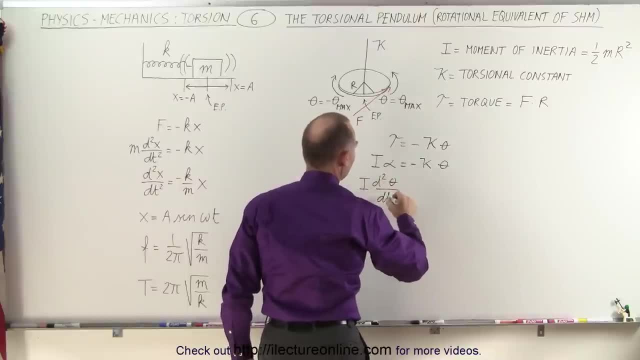 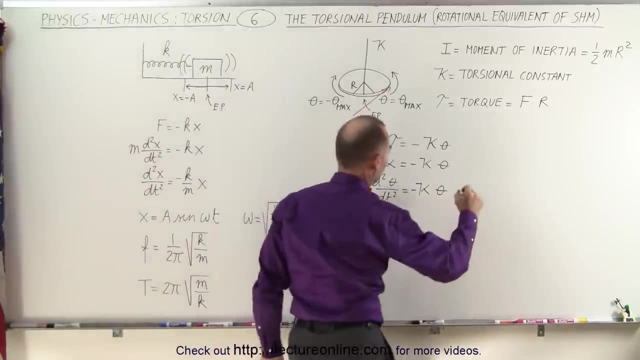 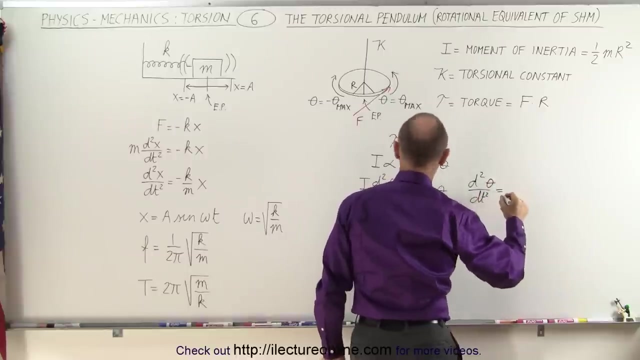 the second derivative of theta with respect to time is equal to minus kappa times theta, and we can then rewrite this in this format- Let me go over here, so don't run out of room- That d square, dt square of the angle, theta is going to be equal to minus. 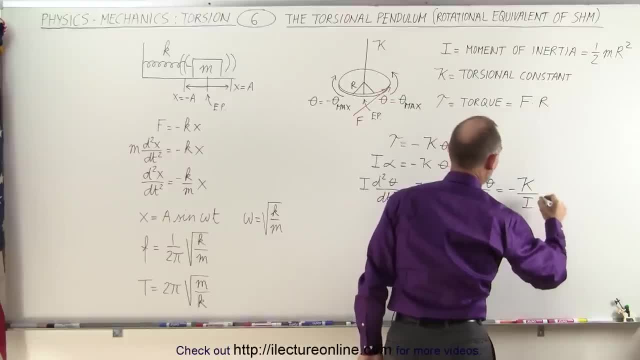 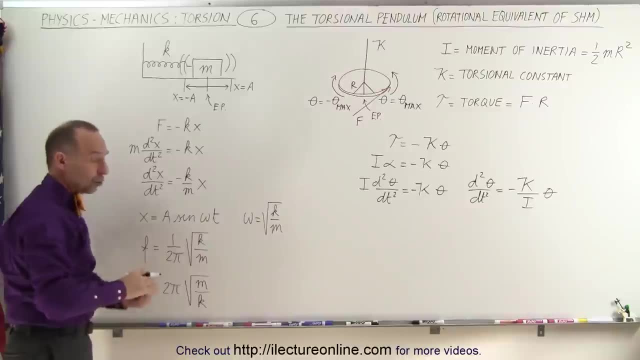 the torsional constant divided by the moment of inertia of the disc times, theta, Just like we did over here. if we solve for this differential equation- and you don't need to know yet how to do that unless you're advanced enough in your mathematics that you do know differential equations- 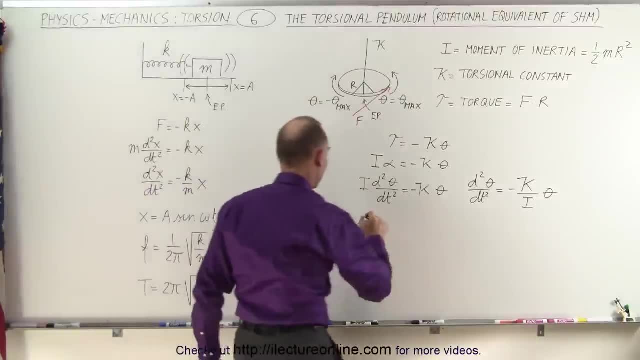 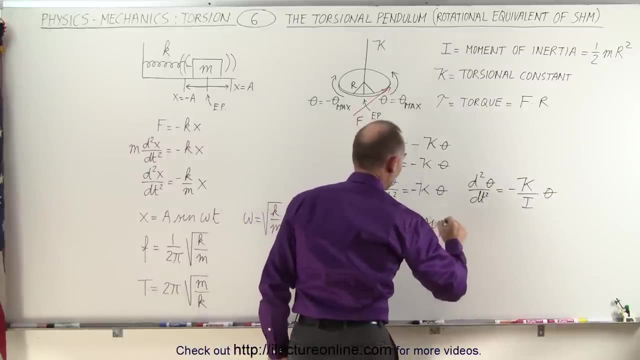 you're going to write it like this- This is the solution to that equation- that the angle theta is equal to the maximum displacement of the rotation times, either the sine or the cosine of omega t. Now, in this case, omega is going to be equal to the square root of kappa, which is the 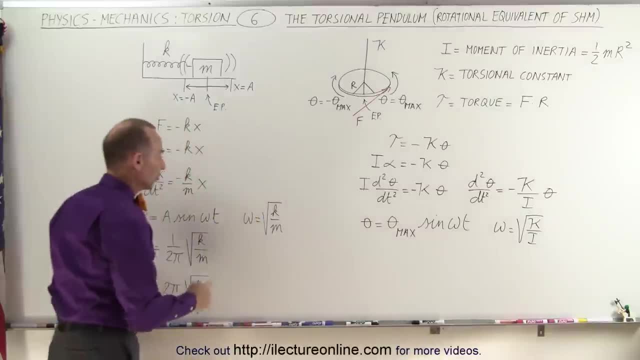 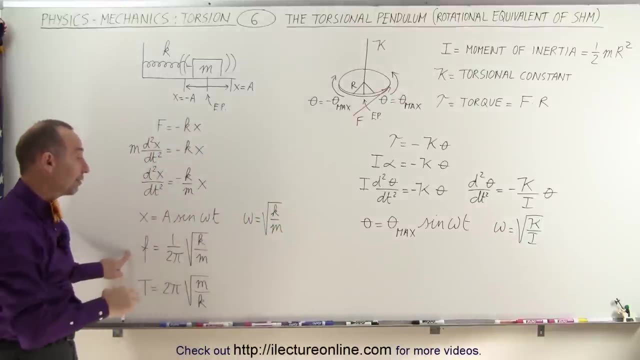 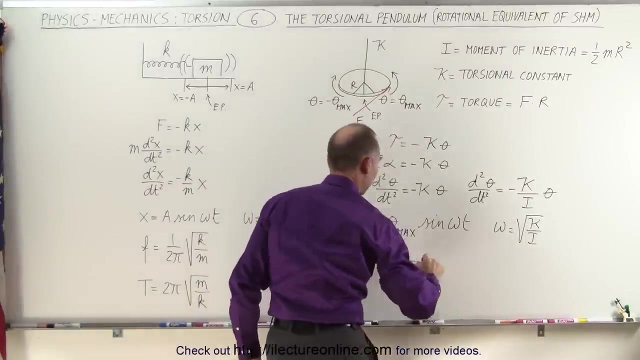 torsional constant divided by the moment of inertia, which is equivalent to the spring constant divided by the mass in this type of system. Now, what we can say is therefore that the frequency, which is equal to 1 over 2 pi times omega, which is equal to 1 over 2 pi times the square root, 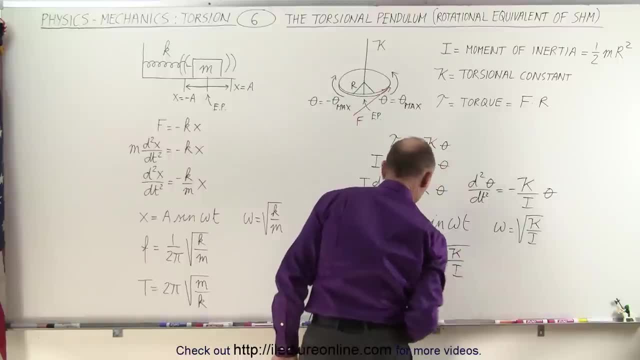 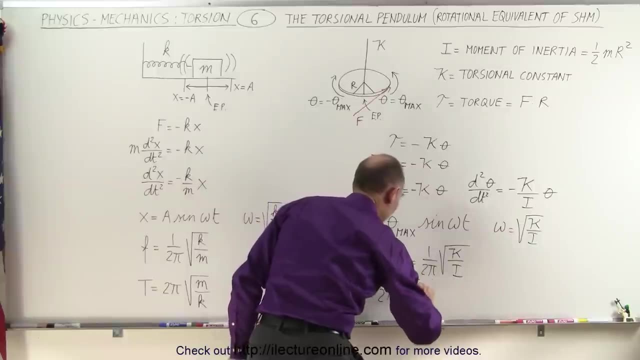 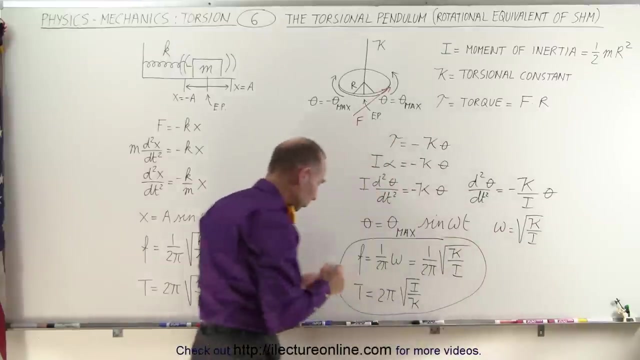 of the torsional constant divided by the moment of inertia. and that also means that the period which is the inverse of that is 2 pi times the square root of the moment of inertia divided by the torsional constant. So here are the two equations you might be very much interested in when you try. 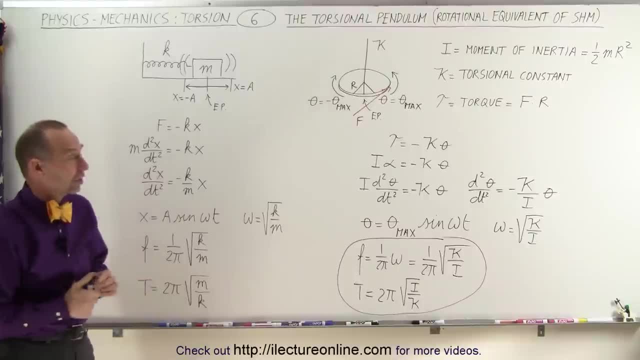 to calculate the frequency or the moment of inertia, the period of oscillation or rotation of what we call a torsional pendulum. So here in this video, all we wanted to do is show you the equivalence between symplomatic motion in a linear fashion. 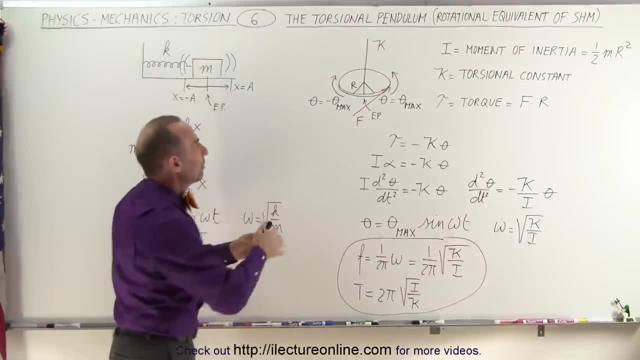 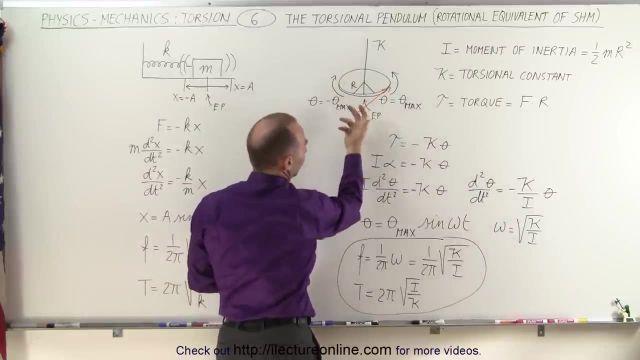 with a mass and a spring which can be calculated. exactly the same for a torsional pendulum, where the displacement will be an angular displacement. instead of the force, we have an applied torque and instead of using the spring constant, we use the torsional constant of the. 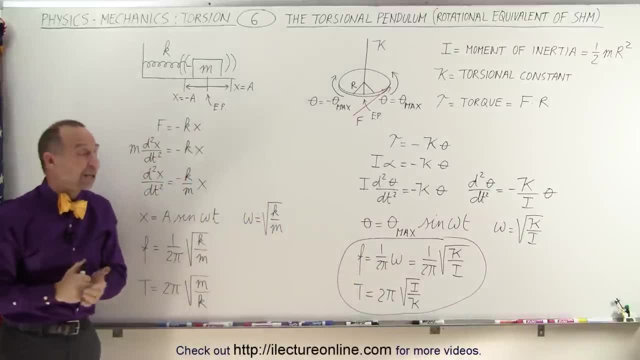 wire or the rod on which it's suspended. So that's how we can see how similar these two approaches are. That's how it's done.